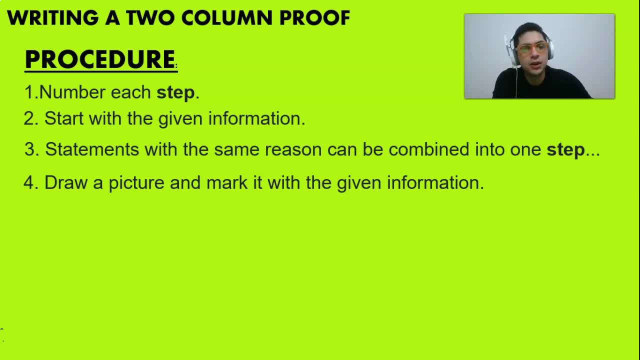 or you can draw a picture or mark it with the given information. So if you guys are given, you can use the one that you're given in order to keep track of the steps of the procedure that you're following. And, last but not least, you must have a reason for every statement, right? so this is 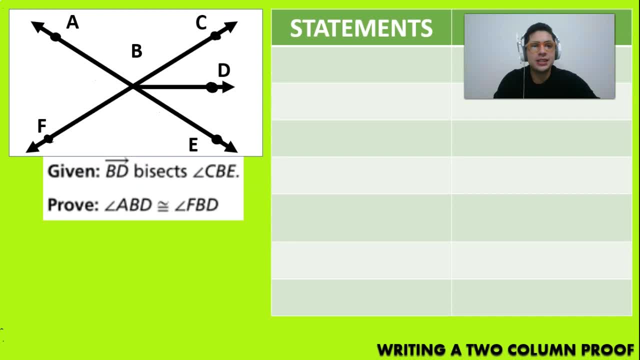 very, very important Now that we know that, let's try tackling this problem here. This is the problem we're going to be doing or working on today. So the first thing is that we're going to see the given. So the given information is that the ray BD, which is this right here, is going to bisect. 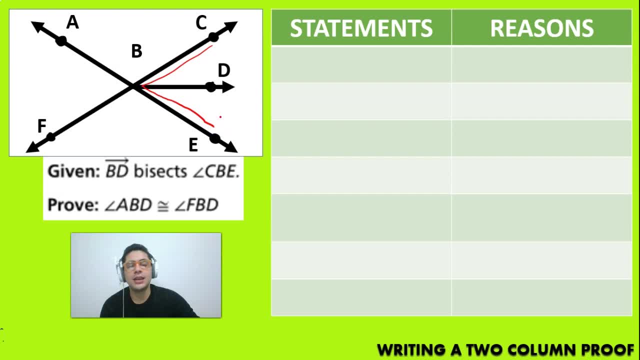 the angle CB. OK, So we have to remember that the definition of bisecting an angle is that this angle is actually going to be similar to this one. OK, But the first thing we have to see is that the ray BD bisects the. 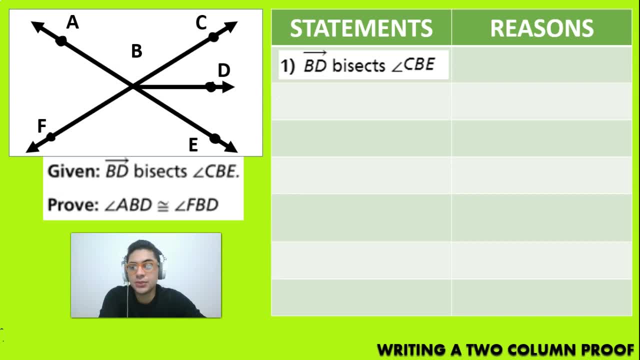 angle. So that is going to be our first statement And when we write down the reasoning, it's going to be given Now, because we know that this angle and this angle are going to be congruent, because they are going to be bisecting. 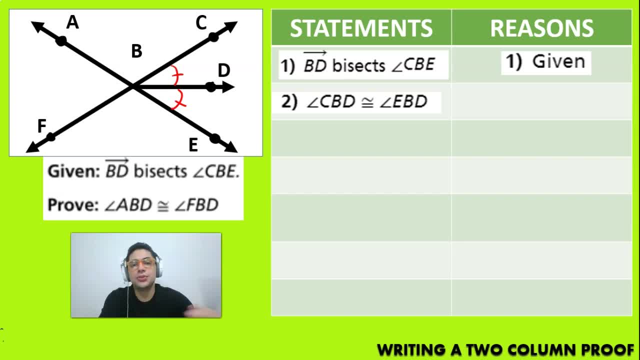 The angle CB E. We are going to write down that the angle CBD is actually congruent with angle EBD, And it is because of the definitions of angle bisector which you have to remember from eighth grade. Now, another thing is that you have the angle A, B, C and you have the angle F, B, E, which are 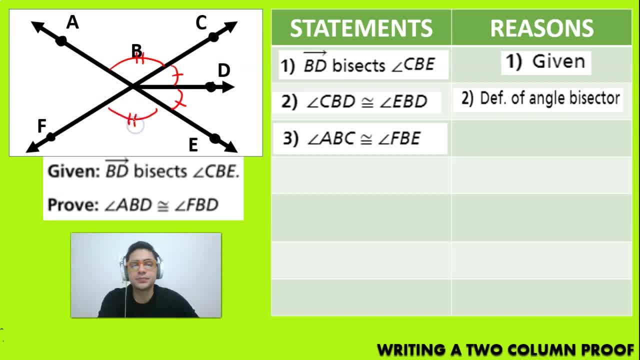 these two, which I'm going to put two tick marks on, And you basically know that they are the same because of the vertical angles theorem. So because they are on opposite sides of the same vertex, you know that they are going to be congruent. Now you know that the 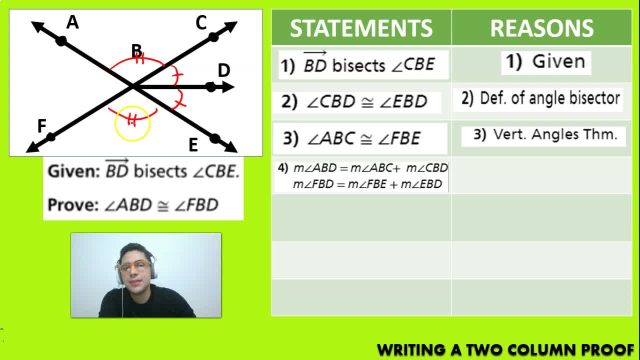 measurement of angle A, B, D and the measurement of the angle F, B, D are going to be equal to the sum of the next two angles, Right. So this angle right here right is going to have a measurement, and then this one is going to have 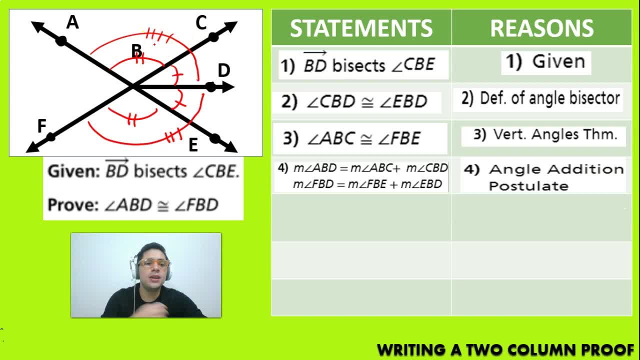 Another Measurement Right. Why? Because the angle addition postulate. I will learn last time. Now we know that the measurement of angle A, B D is equal to the measurement of angle F, B, E, plus the measurement of the angle E B D. Now, guys, if you,